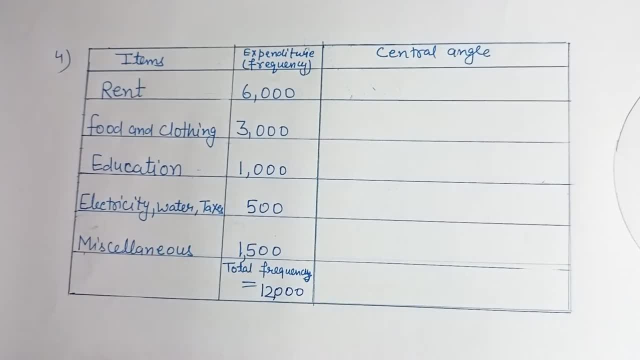 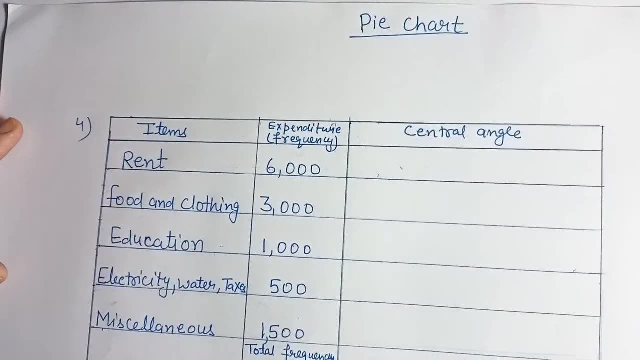 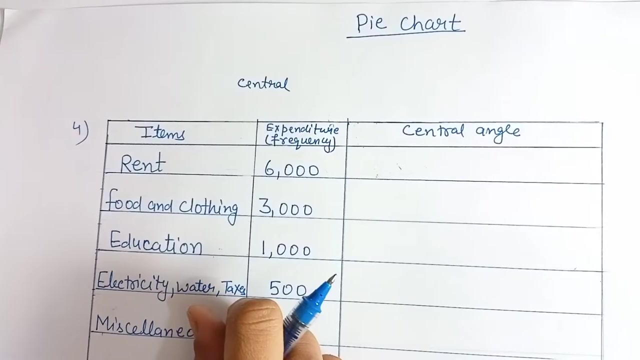 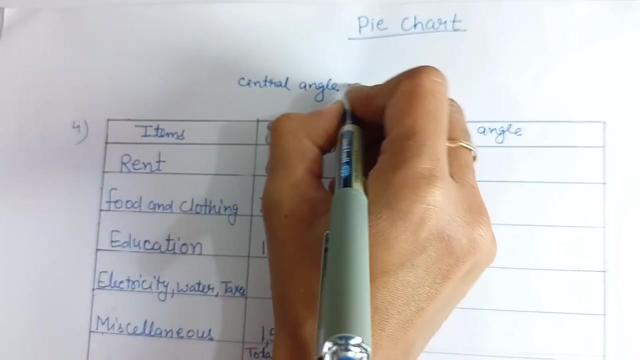 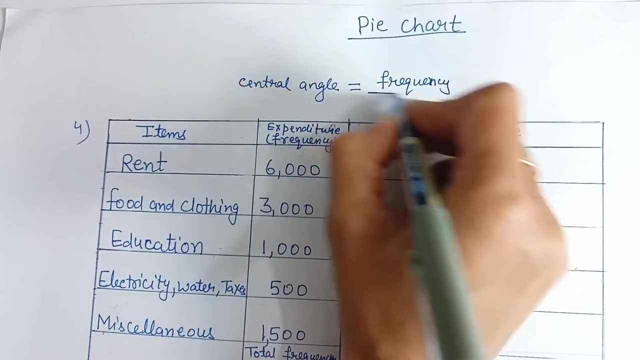 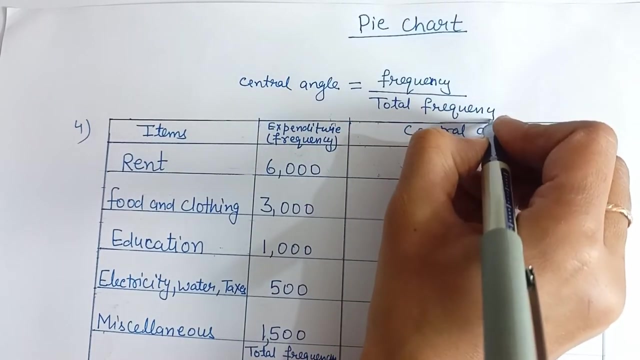 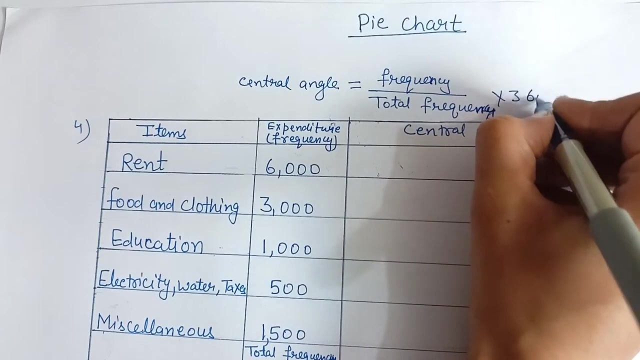 rupees 12,000.. Now we need to find out the central angle for each of the following item. So formula for the central angle is: central angle is equal to frequency divided by total frequency, total frequency multiplied by 360 degree. This is the formula: frequency upon total frequency. 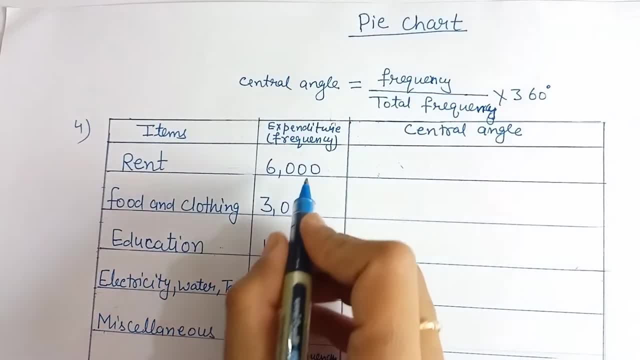 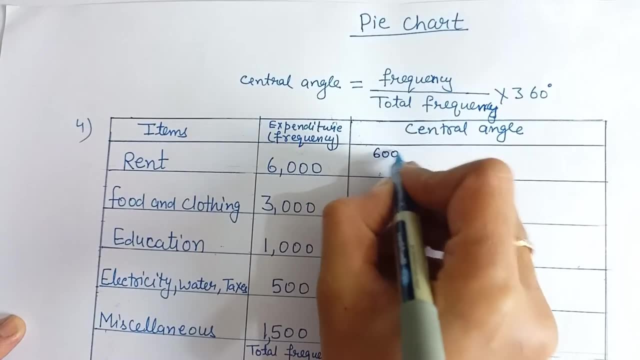 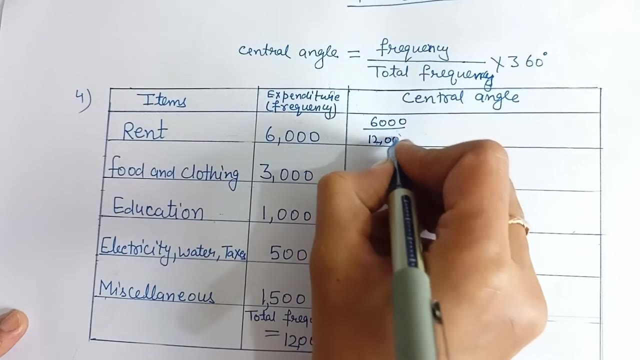 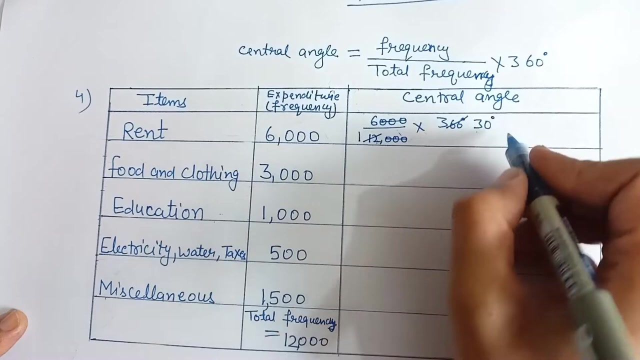 divided by 360 degree. So here frequency is what 6000.? Here frequency is 6000 divided by total frequency, that is 12000.. 6000 over 12000 multiplied by 360 degree, So 30 cancelled with 30.. Now 12 ones are 12, 12, threes are 36 and 10. 30 degree: 30 multiplied by 6 is 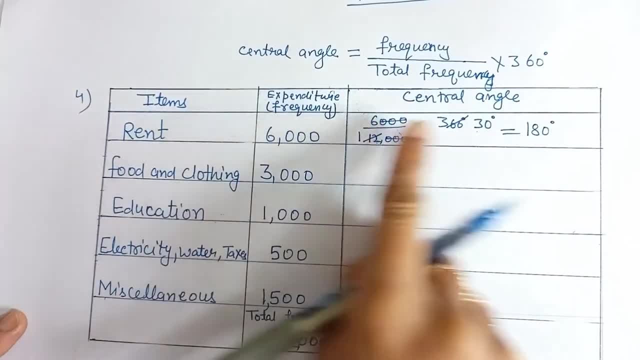 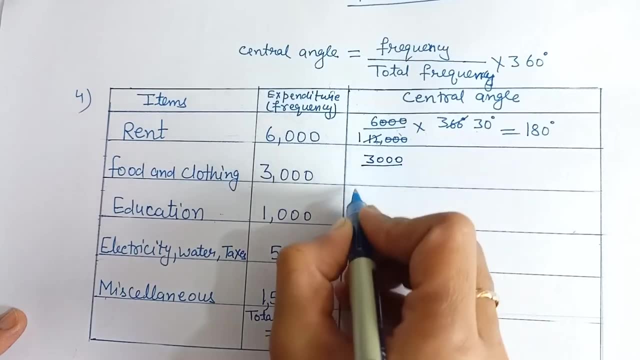 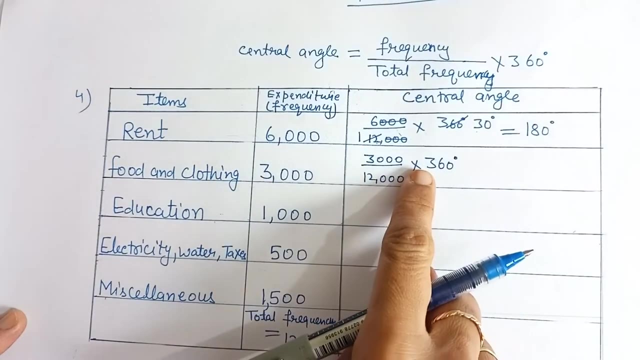 180 degree. So central angle for rent is 180 degree. Now for food and clothing. what is the frequency here? 3000.. 3000 and total frequency 12000, multiplied by 360 degree. 360 degree because that sum. 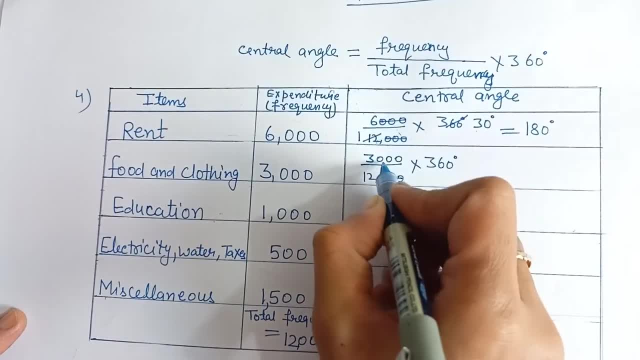 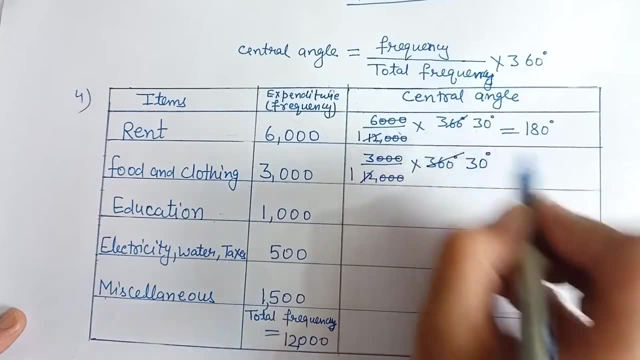 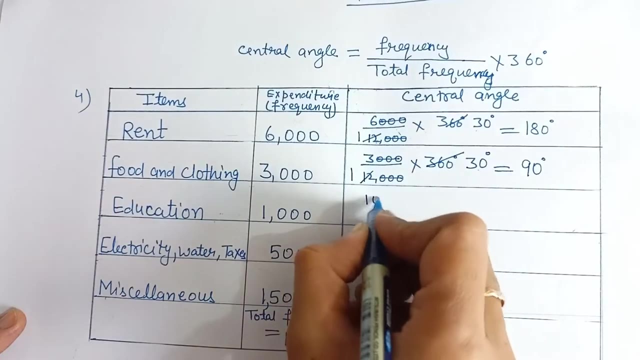 of all the angles in a circle is 360 degree. That is why 360, 30 cancelled with 30, 12 ones are 12, 12. threes are 36, 10, 0 degree. Now 33 is a 90 degree For education frequency. is 1000.. So for food and clothing, what is the frequency here? 3000 multiplied by 12, 12, threes are 36 and 10. 30 degree, Now 33 is a 90 degree. For education frequency is: 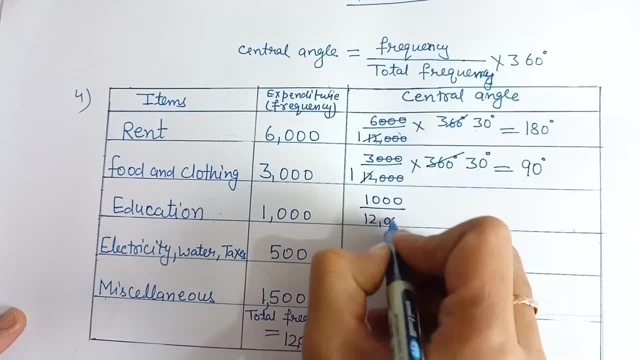 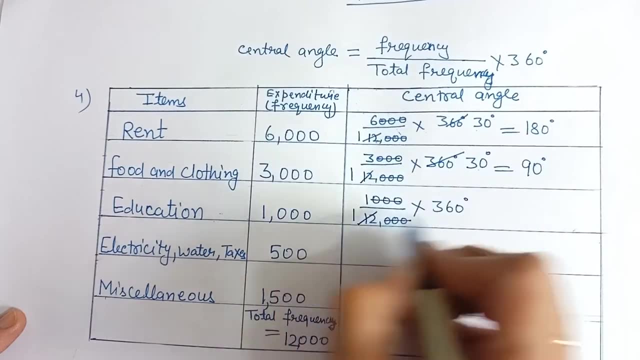 1000, total frequency 12000 multiplied by 360 degree. So 300 cancelled with 30.. 12 ones are 12, 12, threes are 36 or 0, 30 degree. So 30 degree angle. Central angle for education, Angeles audio. 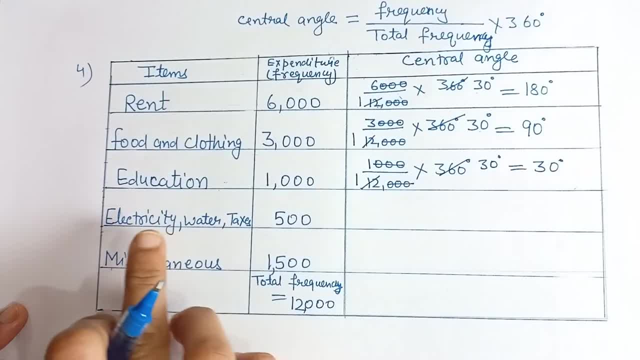 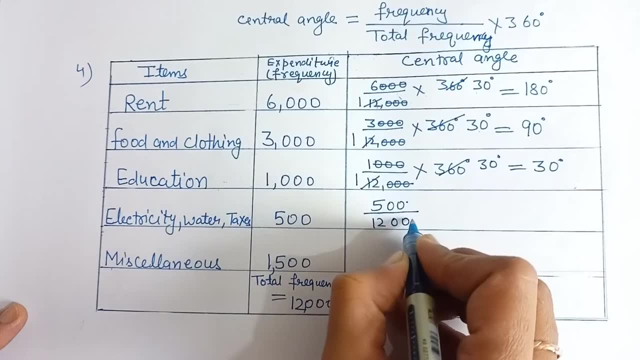 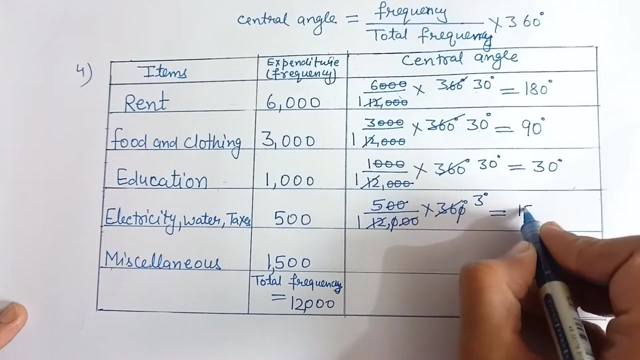 cut in pauses is 500 multiplied by 360 degree. ca 2: 0. cancel with 2: 0, 1: 0 from here. now 12 ones are 12, 12 threes are 36, now 5 threes are 15 degree. 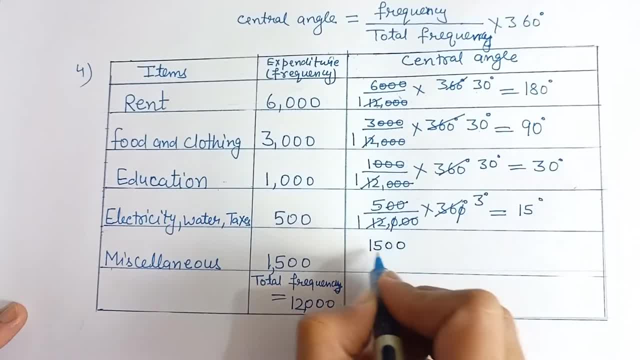 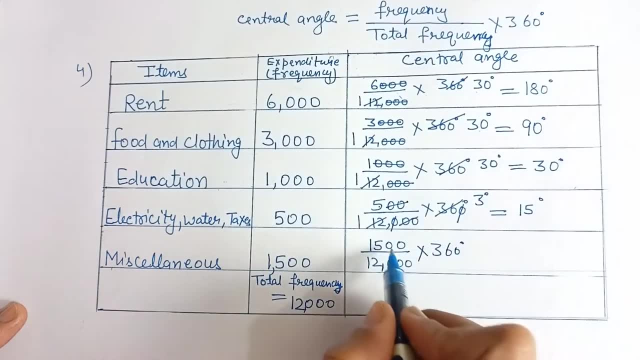 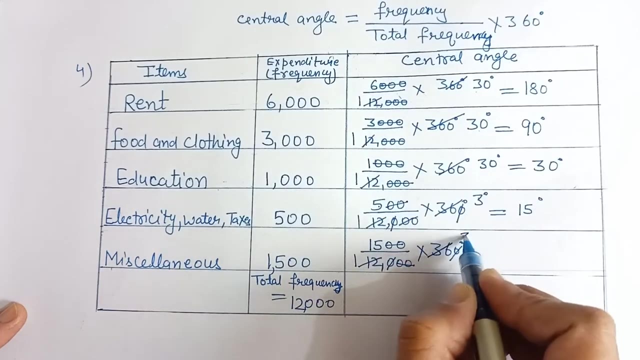 For miscellaneous frequency is 1500,. total frequency is 12000, multiplied by 360 degree: 2: 0. cancel with 2, 2, 0, 1, 0. from here now, 12 ones are 12,, 12 threes are 36,, 15 threes are 45, because degree, we have that degree. 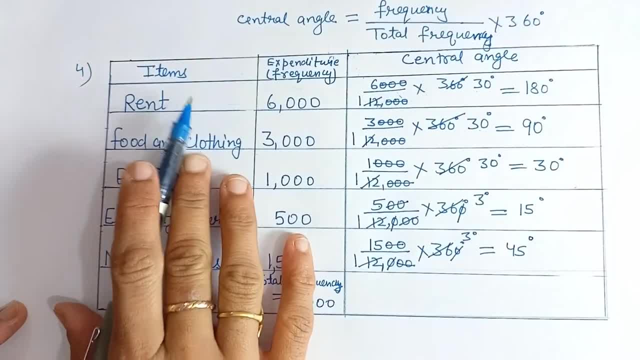 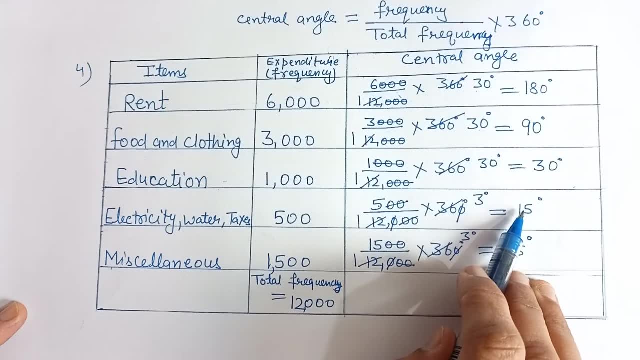 So we have already calculated. the central angle for rent is 180,, food and clothing 90 degree. for education it is 30 degree. electricity, water intake is 15 degree. for miscellaneous it is 45 degree. Now we will draw. 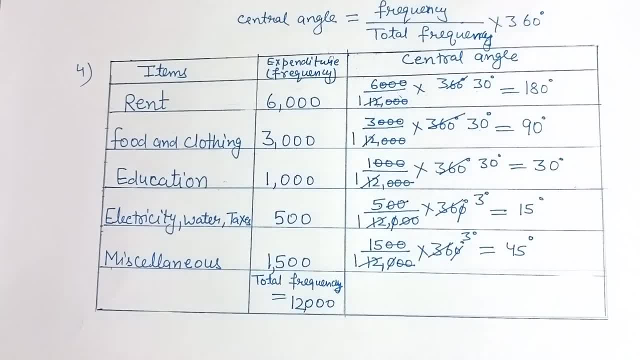 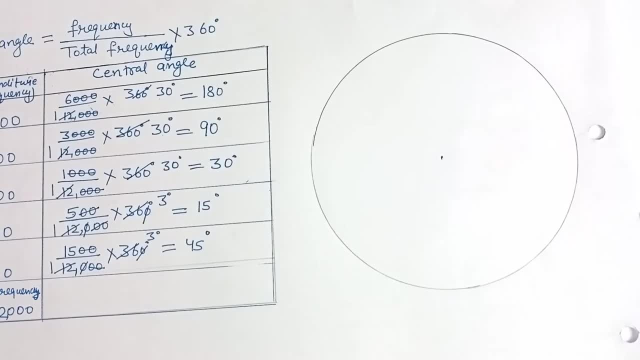 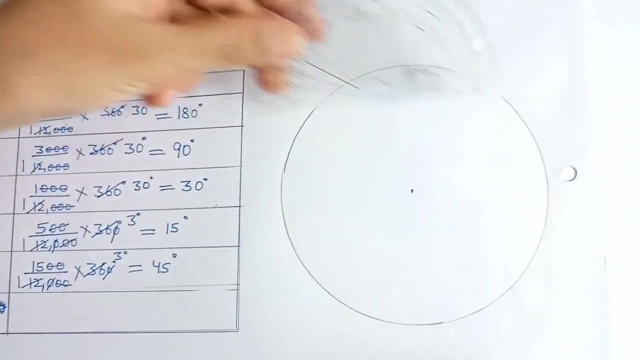 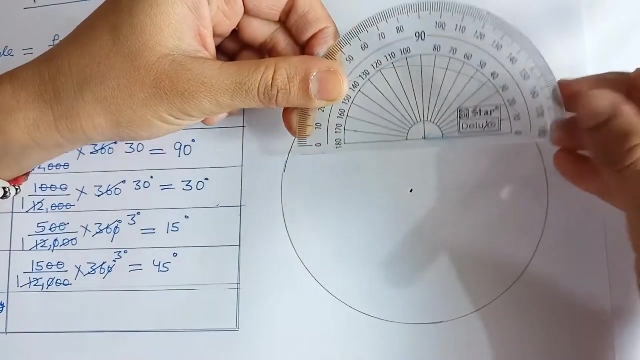 This, these central angle in a circle and that we will call pie chart. so first draw a circle. now, the first angle is 180 degree. that is for rent, as we know that 180 degree is a straight line. so how we will draw, we will coincide. this point and the center of the circle must coincide. it is a straight line. 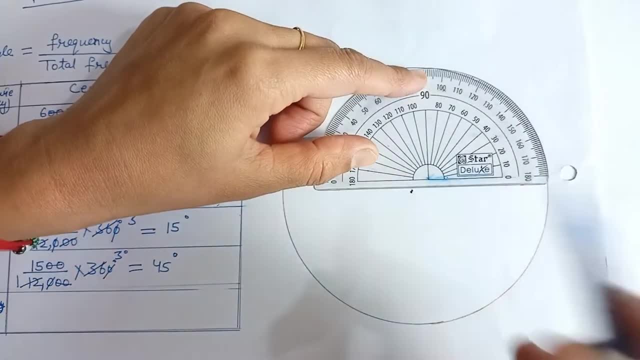 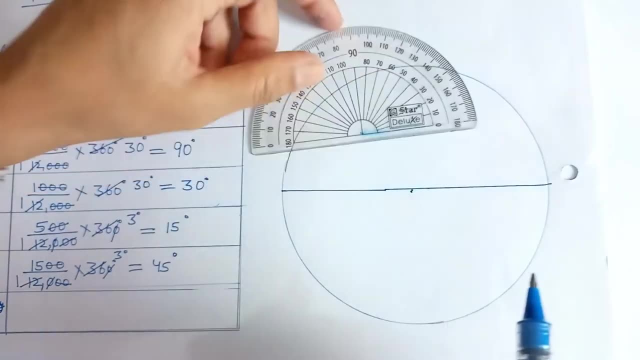 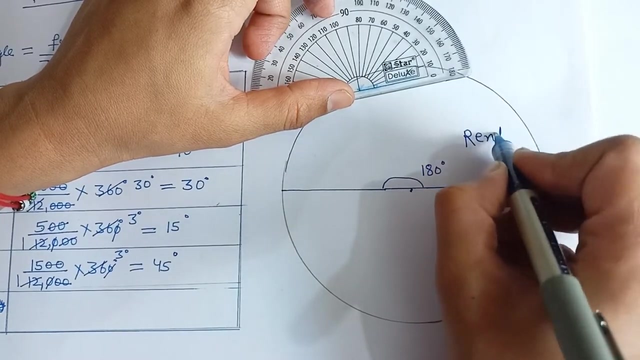 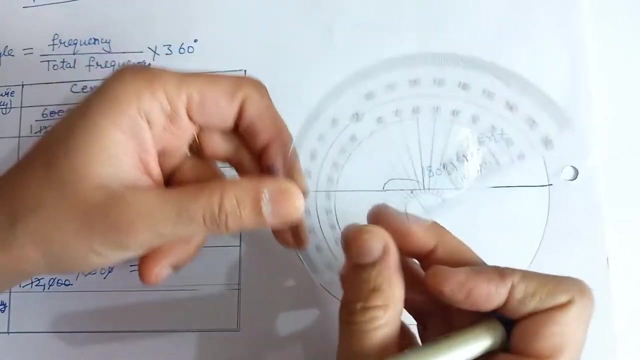 So we can draw. So we can draw a straight line without measuring. draw a straight line, okay. so this is 180 degree from here to here. this is 180 degree. and for what this is? for rent again now, food and clothing, it is 90 degree. now this point and this point will coincide and the 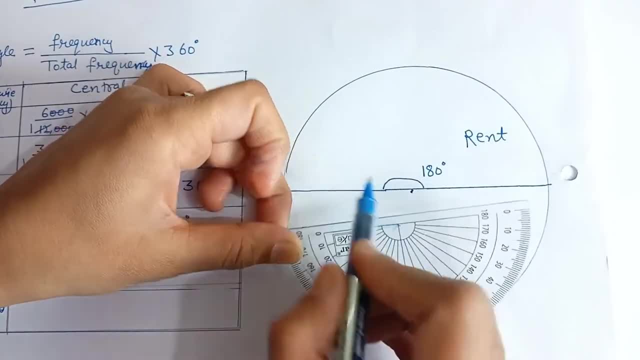 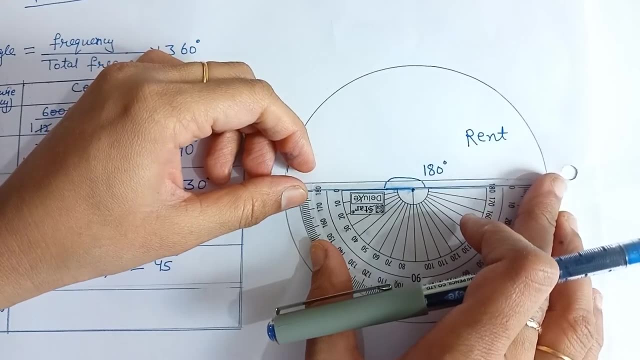 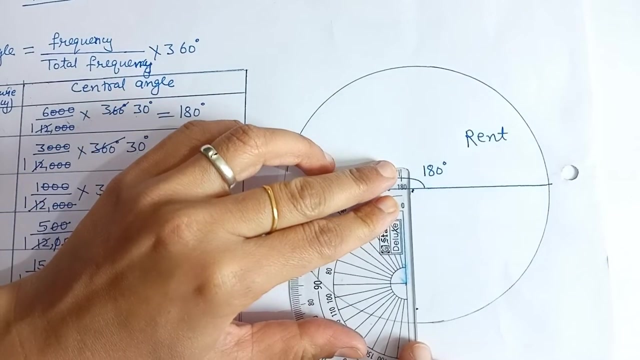 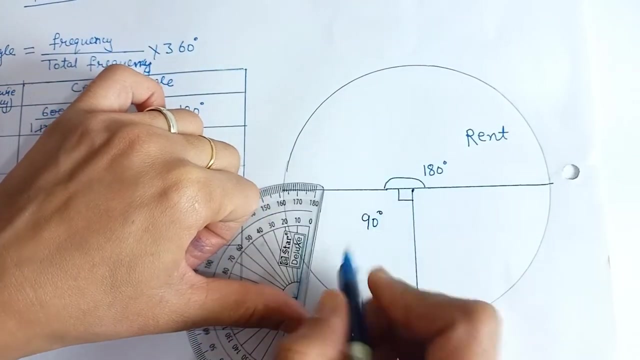 like this: the zero degree line will coincide with this line and this point with this, and both line coincide over each other. now, where is 90 here, here? so we will join these two points. this is 90 degree. 90 degree for what? food and clothing. 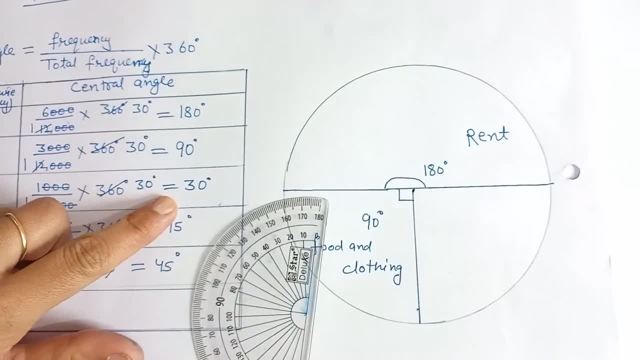 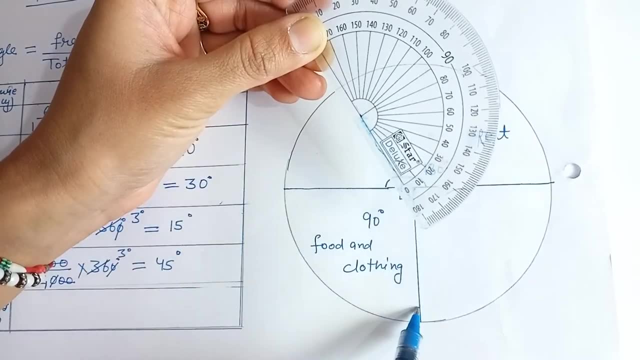 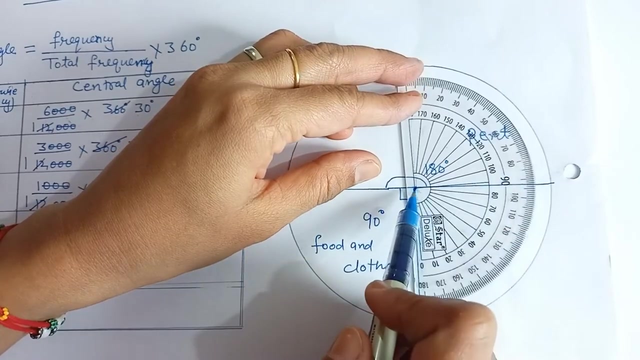 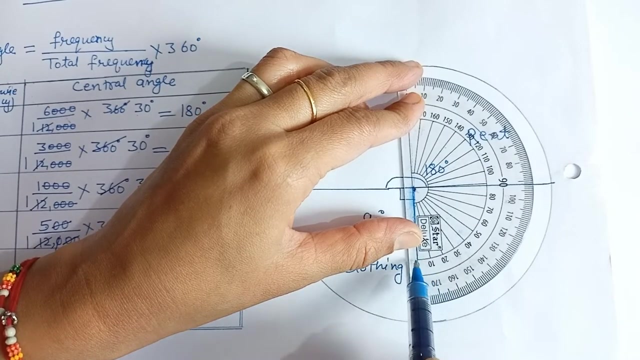 Next is education angle is 30 degree now. now this point will coincide with this point and just zero degree line will be over this line. so place your protector like this, so that this point will coincide with the center and this line, with zero degree line over this line. so, 30 degree, 0,, 10,, 20 and 30, here it is 30. 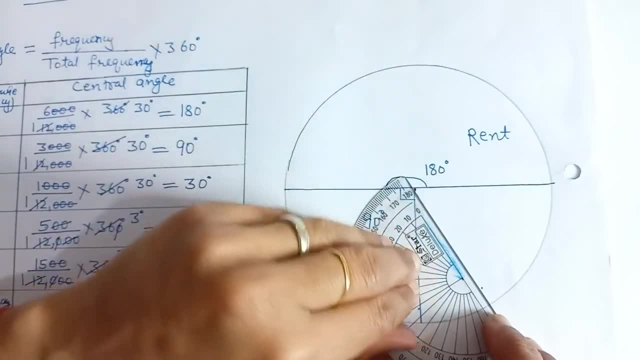 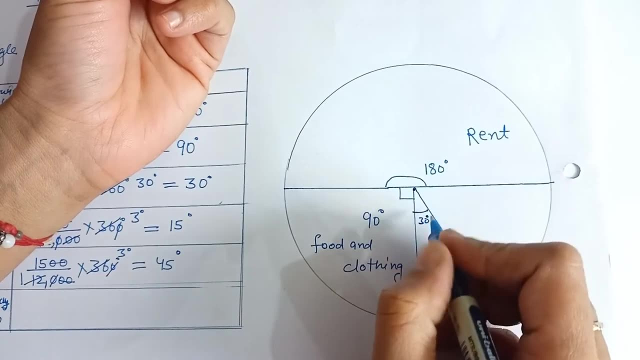 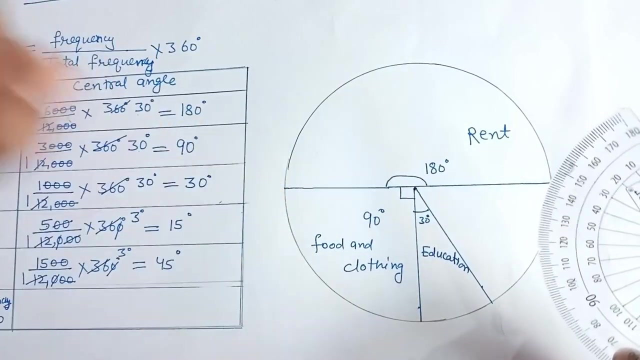 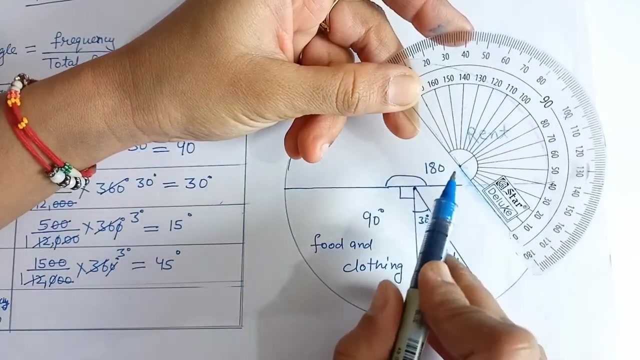 Now join this dot to the. this is our 30 degree angle. this is for education. Next is electricity, water and texas, and angle central angle is 15 degree. again, what we will do, We will coincide this 0 degree line over this line, 0 degree line over this line, and this: 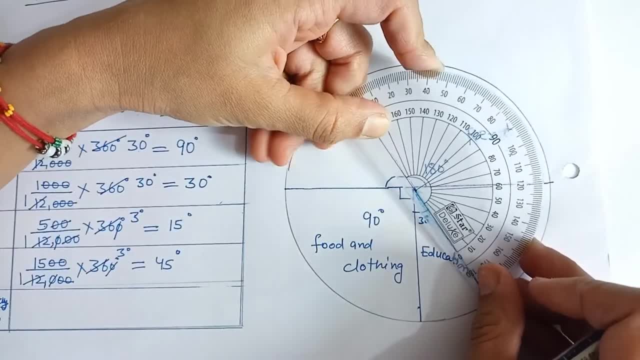 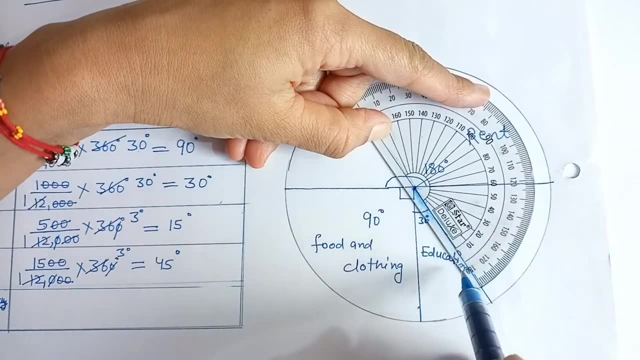 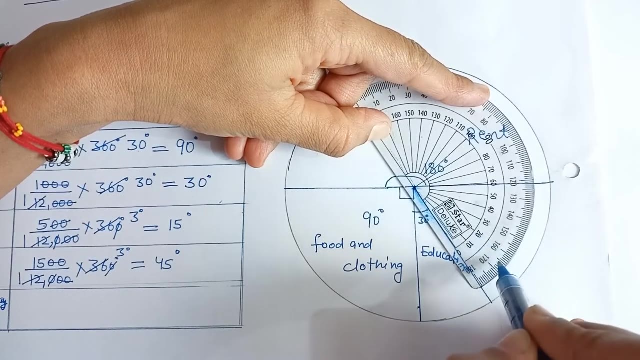 dot at this point. so place your d like this, so that this point and the center of d must coincide, and the 0 degree line over this line, Now 15 degree. this is 0, 10, 20, so in between 10 and 20 there exists line that is of 5,. 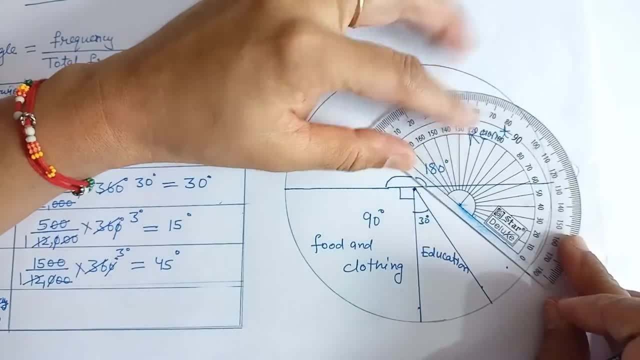 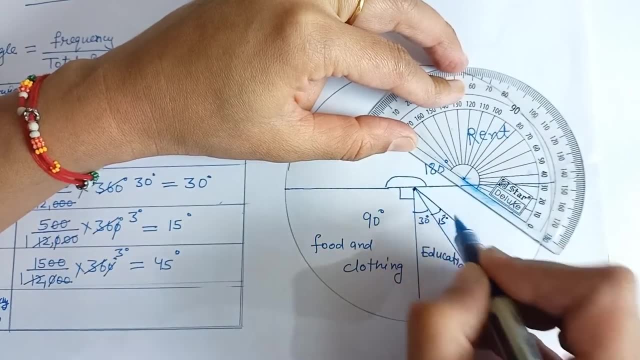 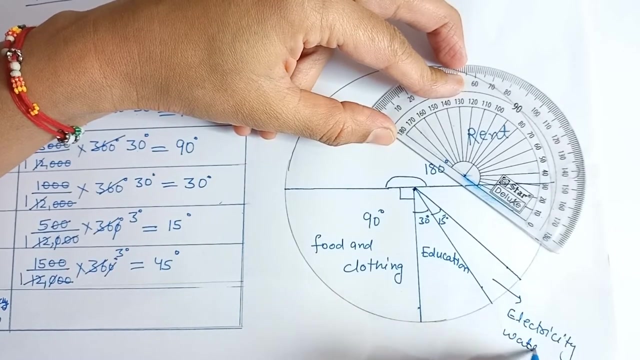 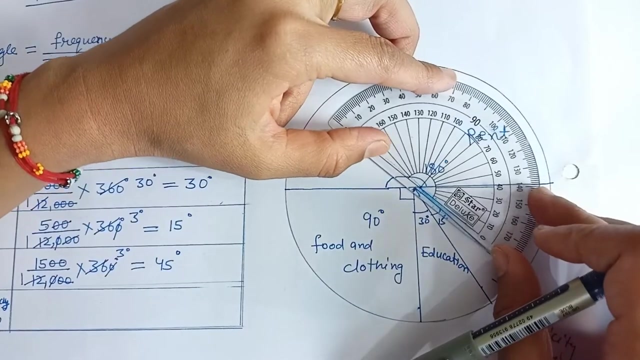 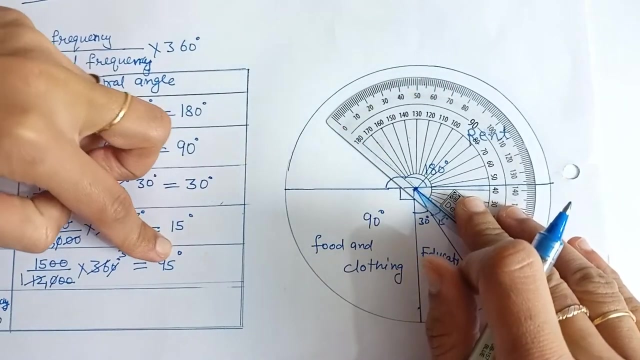 so 10 or 5,, 15.. Now join these two. this is 15 degree And this is for electricity, water and texas, and this remaining angle will be of 45 degree. you can measure, see this is already of 45 degree. this is because the sum of all the 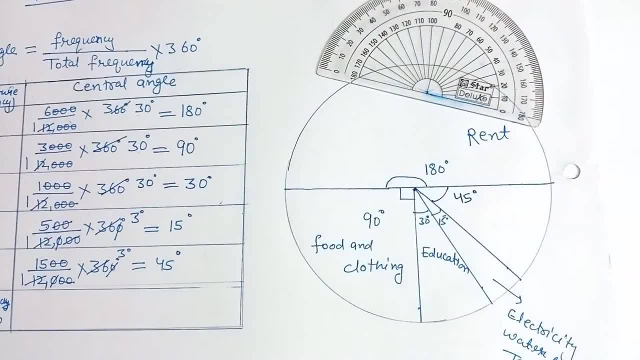 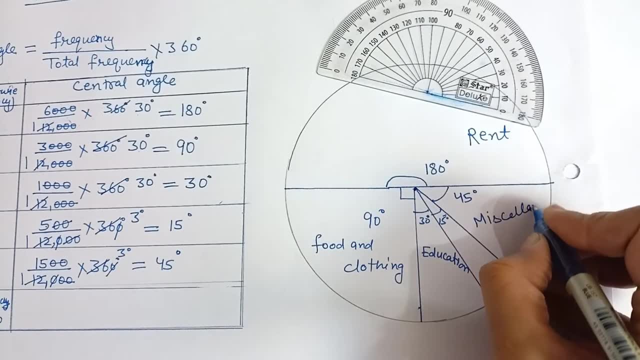 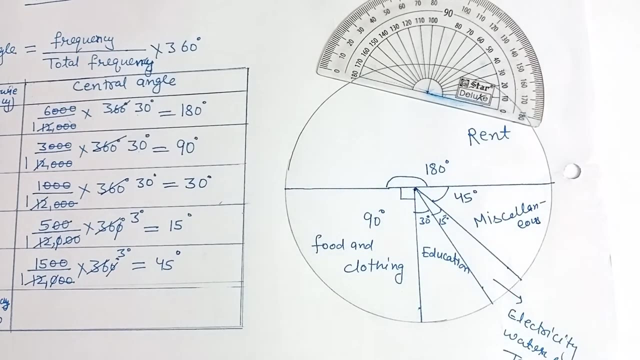 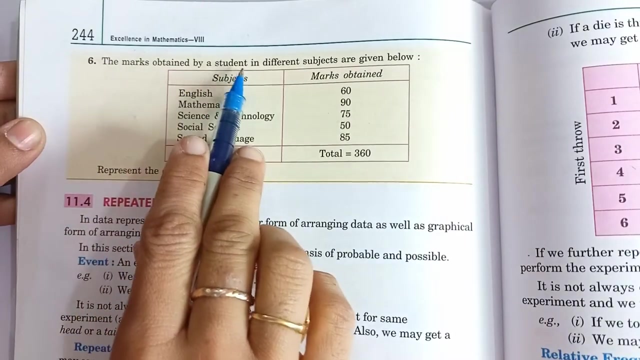 angle is of 360 degree. that's why it remain only of 45 degree. And for what? For miscellaneous. so the pie chart for this question is complete, So let us do one more question of pie chart. question is the marks obtained by a student? 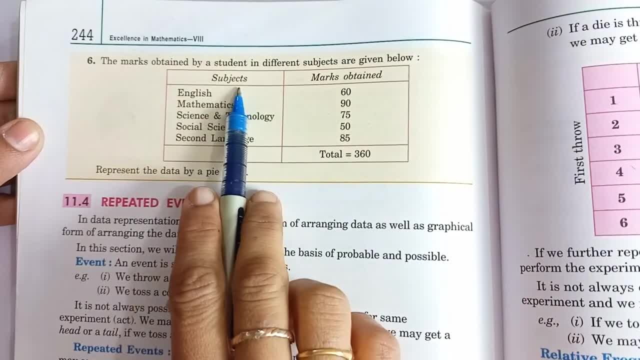 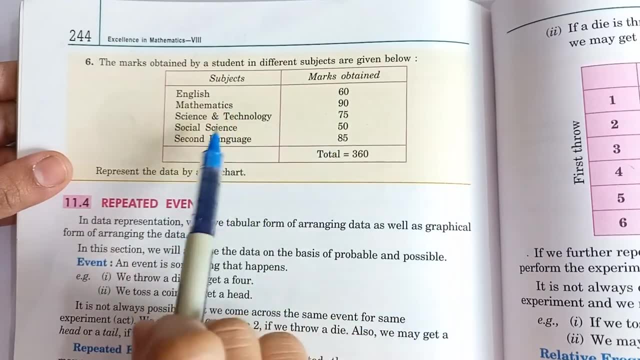 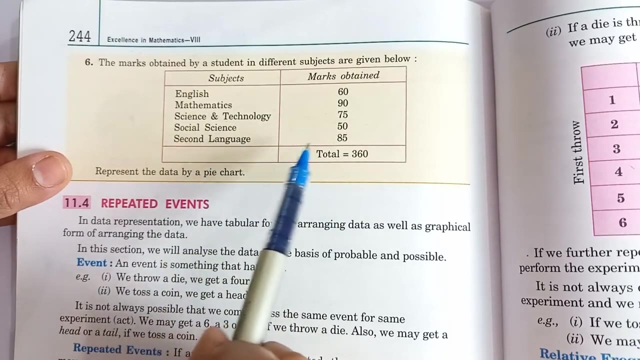 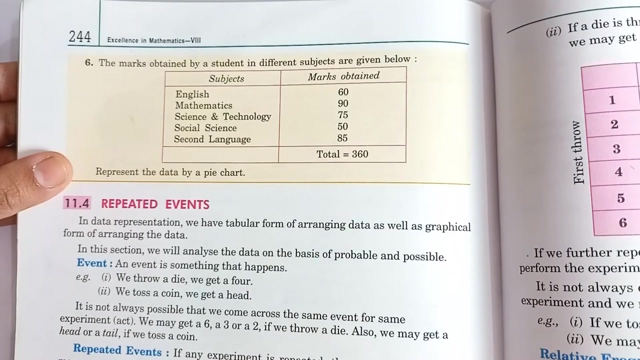 in different subjects are given below. In subject, these are the subject name and these are the marks obtained in English: 60 marks. mathematics: 90.. Science and technology: 75,. social science: 50 and second language: 85.. Here in this question, the total of all the marks is means. total of frequency is also. 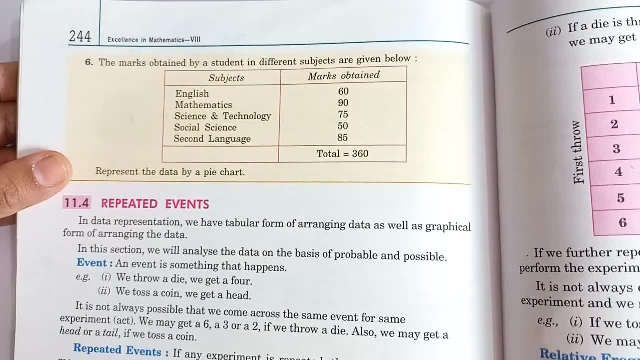 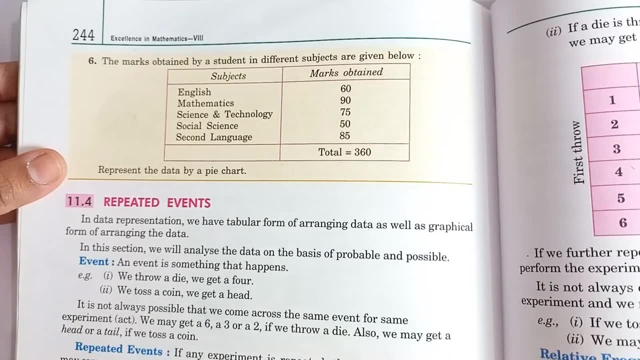 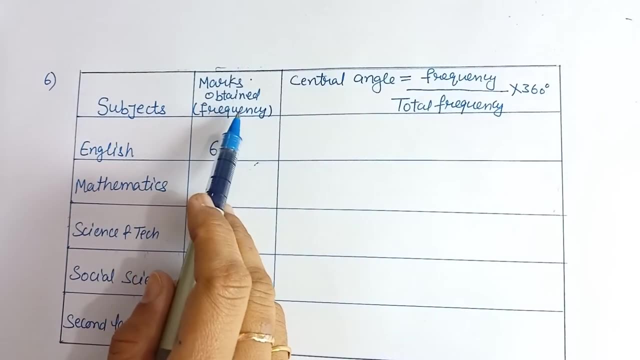 given that is 360.. So we need to find out central angle for each of the subject. then we will draw pie chart. Let's start So. this is the table Here: subject's name: marks obtained. this is also called frequency. 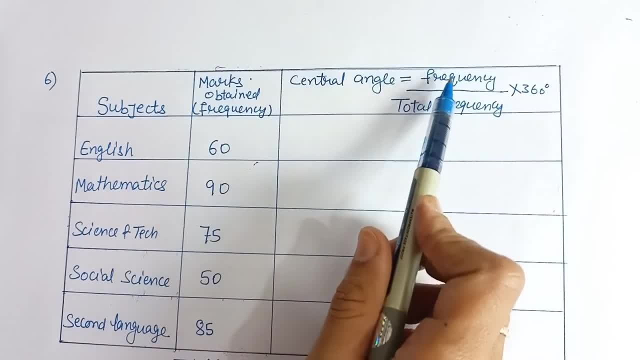 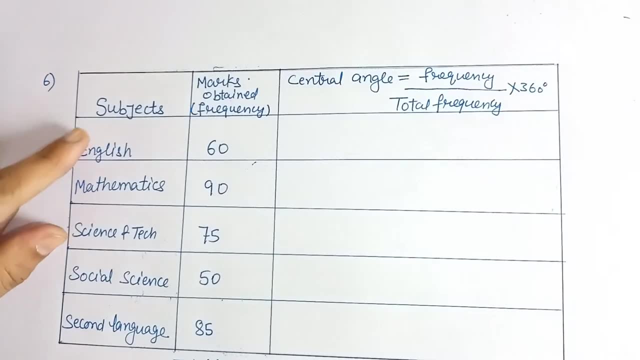 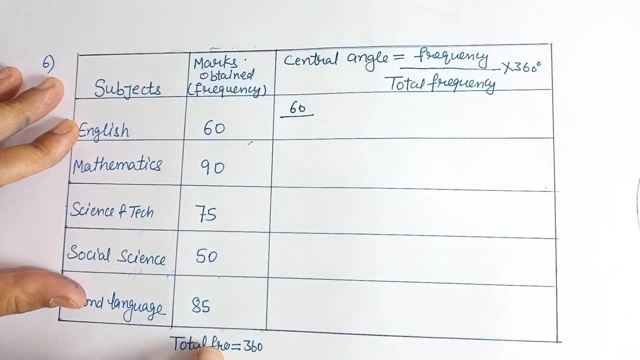 Here we will find out the central angle. the formula for central angle is frequency divided by total frequency multiplied by the 360 degree. So for English the frequency is 60 and the total of all the marks is 360, means total frequency is 360.. 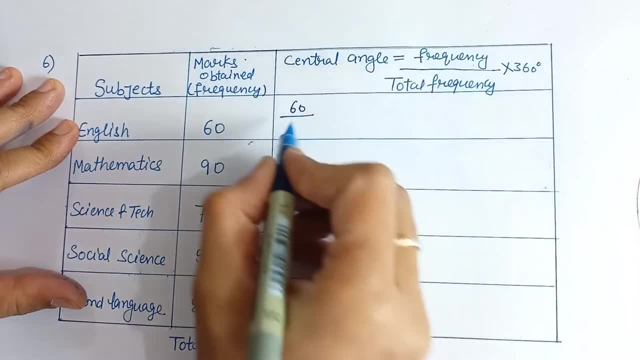 So formula central angle is frequency divided by total frequency. So this is the table Here. subject's name marks obtained. this is also called frequency. That means 60 divided by 360, multiplied by 360 degree: 360 ones are 360, 360 ones are 1 degree. 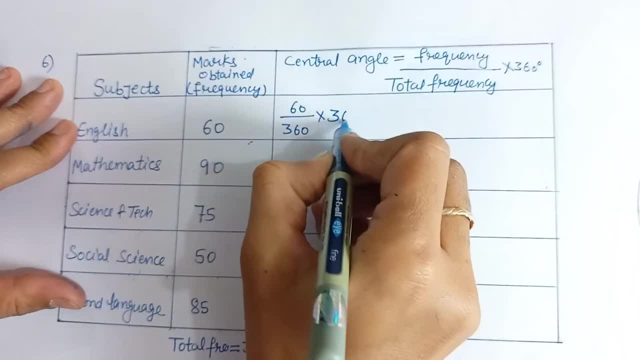 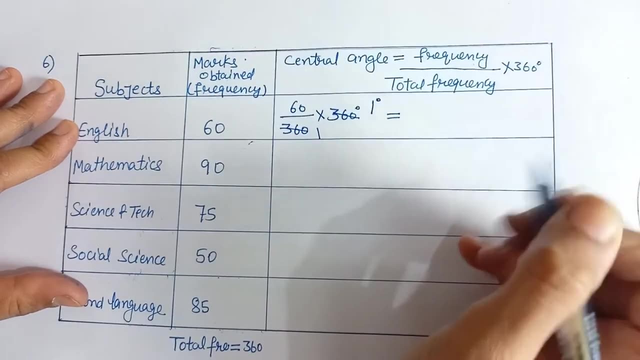 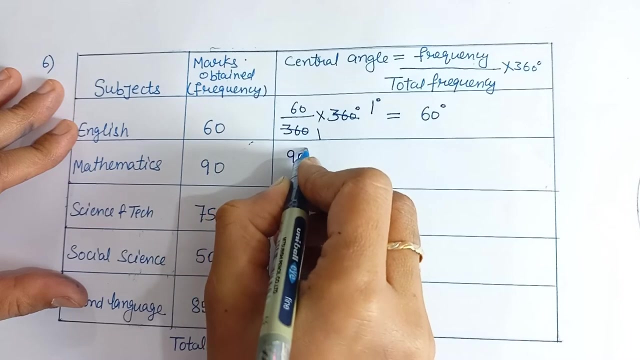 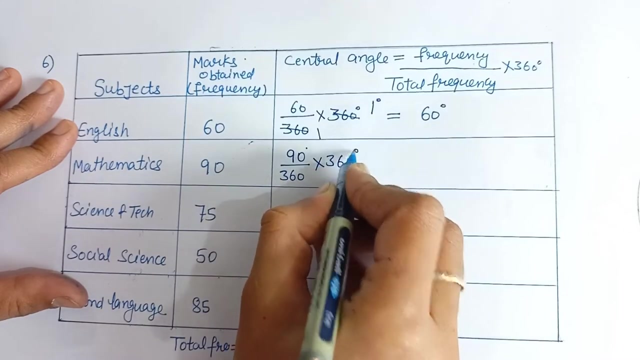 Because this is a degree. that's why we will write degree 60 into 1 degree is 60 degree. For mathematics frequency is 90 and total frequency is 360 multiplied by 360 degree. Again, this cancelled out. Only 1 degree will remain here. 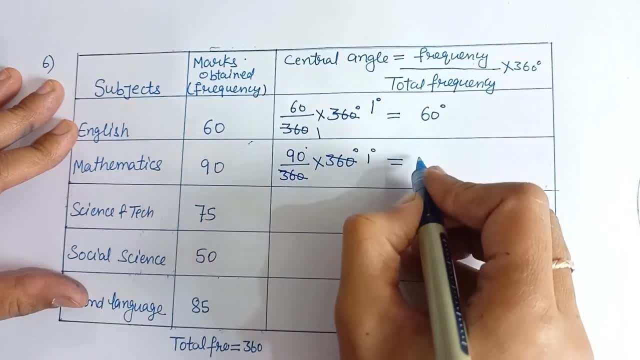 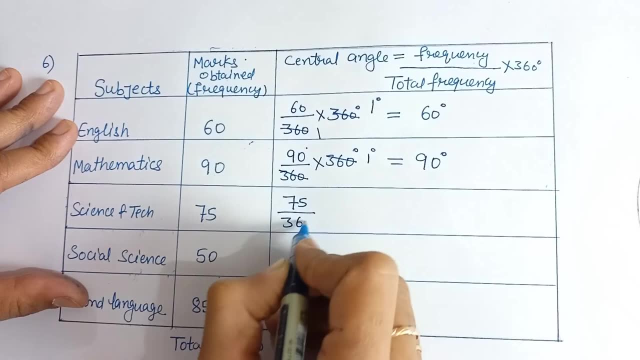 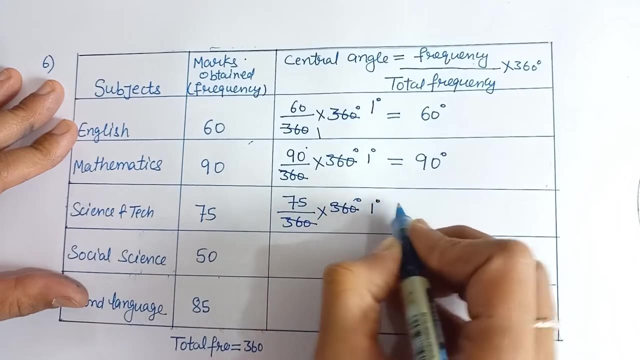 360 ones are 360, so 1 degree into 90 is 90 degree, Next is 75.. Upon total value, that is 360 multiplied by 360 degree, 360 ones are 360,. 360 ones are 360,, 75 ones are 75 degree. 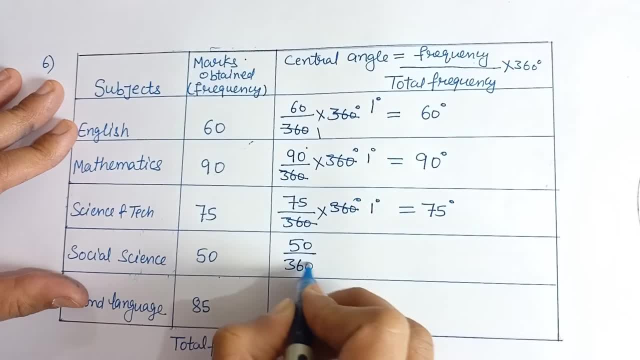 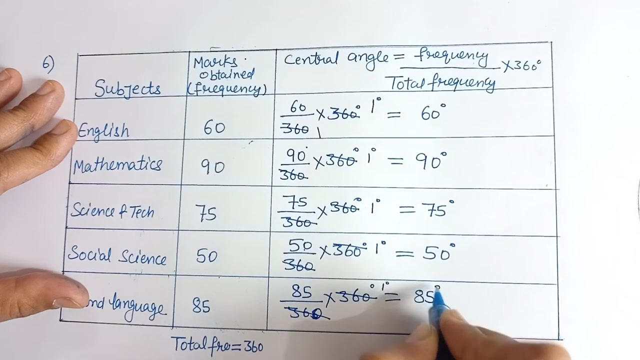 Next is 50 over 360 multiplied by 360 degree. Next is 50 over 360.. Next is 50 over 360 multiplied by 360 degree. 360 ones are 360, 360 ones are 360.. 50 into 1 degree is 50 degree. Last is 85 upon 365 multiply 360. This is 360 into 360 degree. Get cancelled, only 1 degree remain here. 1 degree into 85 is 85 degree. 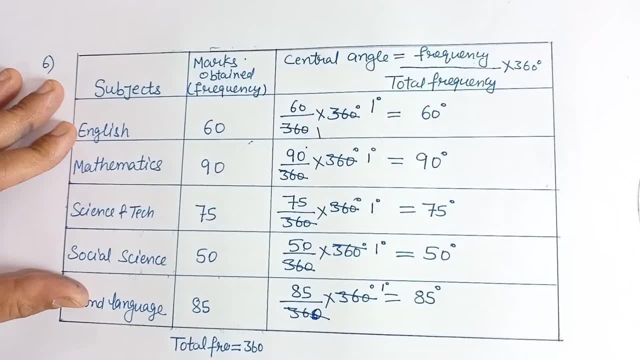 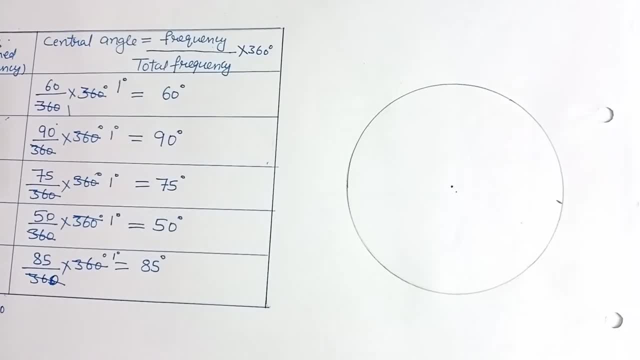 Now we will draw the pie chart of this given data. So for that we need to draw a circle. We have already drawn a circle. Now the first for English mark, central angle is 60 degree. With the help of protector, we will draw 60 degree angle. 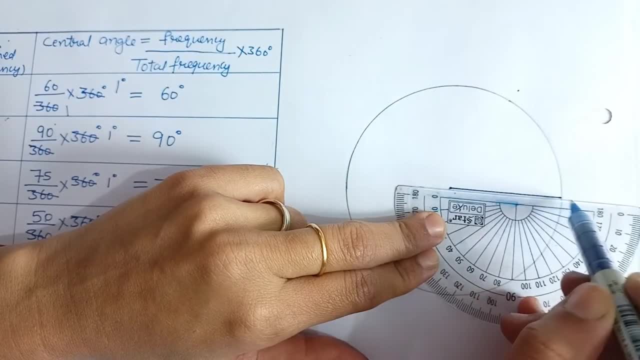 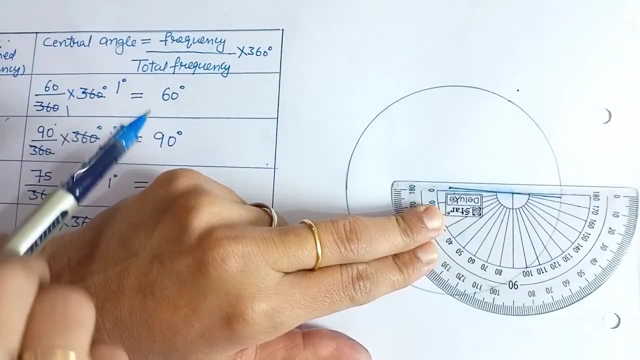 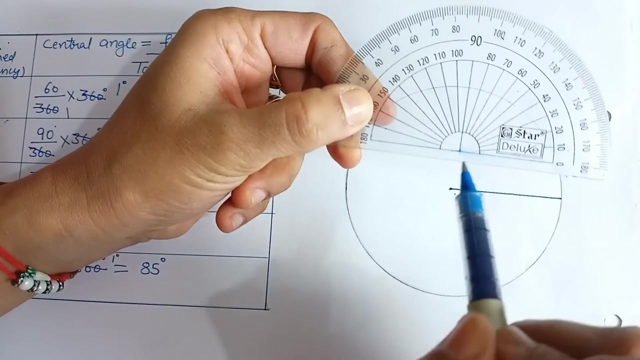 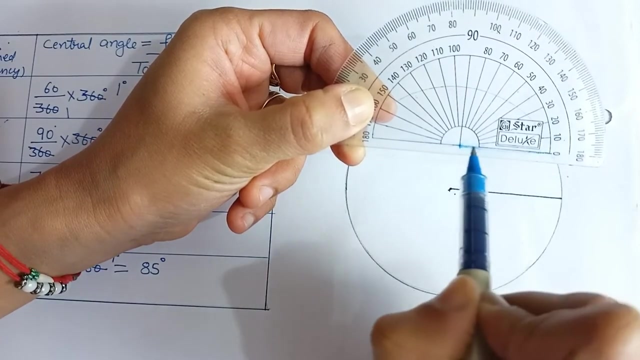 First, we will draw a line joining center of the circle to any point on the circle. Now, what we will do, we will draw. we have to draw angle 60 degree, Central angle, that is central angle for English. So for that we need to coincide this point to center of the circle and this 0 degree line to this line. 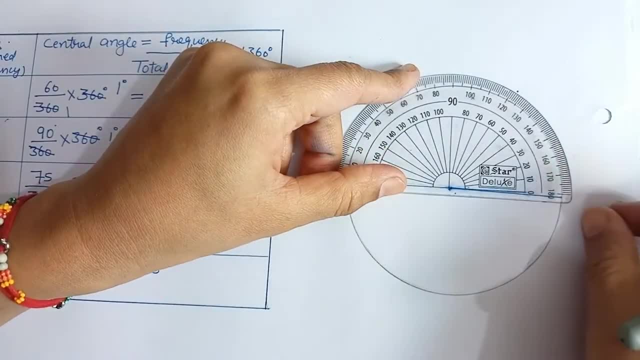 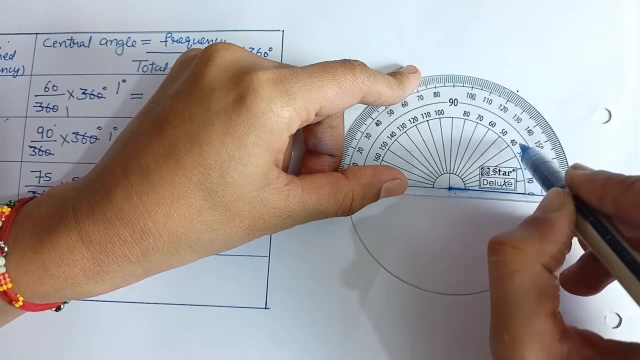 So that this point overlap over the center of circle and this 0 degree line over the radius, Now 0.. 10,, 20,, 30,, 40,, 50,, 60. Here is 60. We will write a dot here And now we will join. 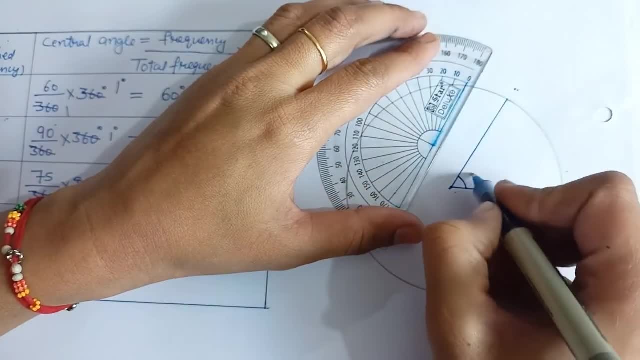 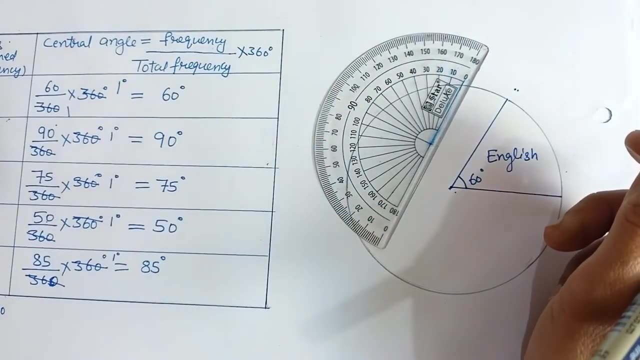 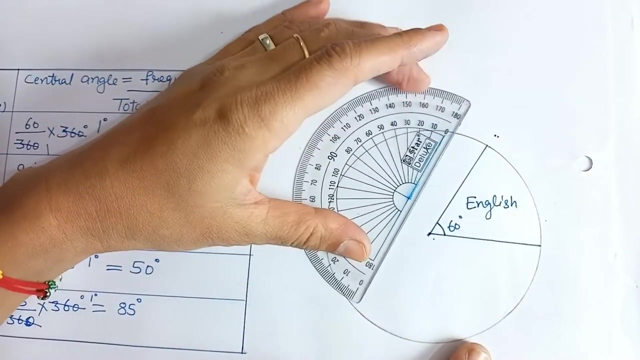 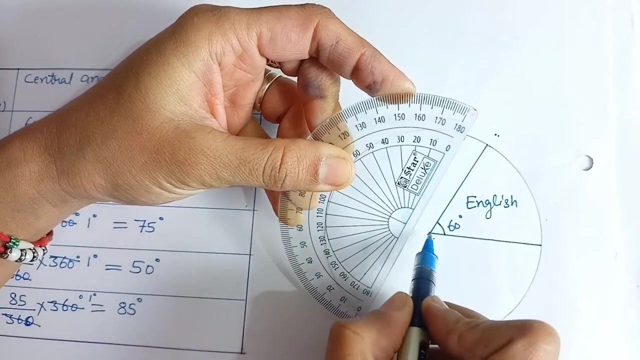 We will not go out of the circle. So this is 60 degree And this is for English, After English mathematics, After English mathematics, angle is 90 degree. So now we will shift our compass like this. We will again the same, We will follow the same rule. This point must coincide: center of the circle and this 0 degree line. over this line. 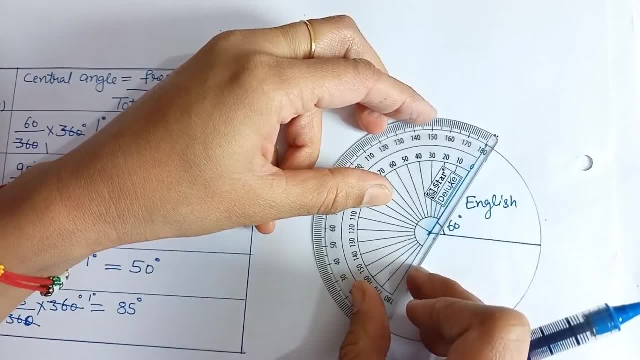 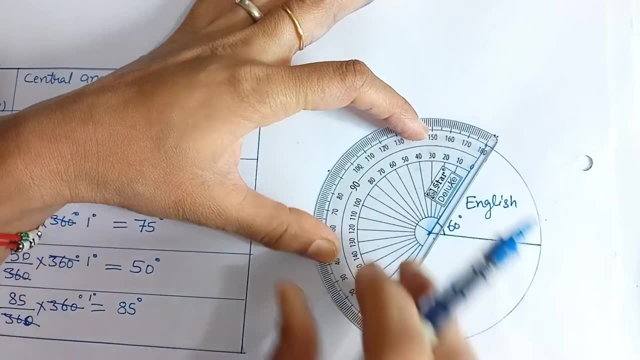 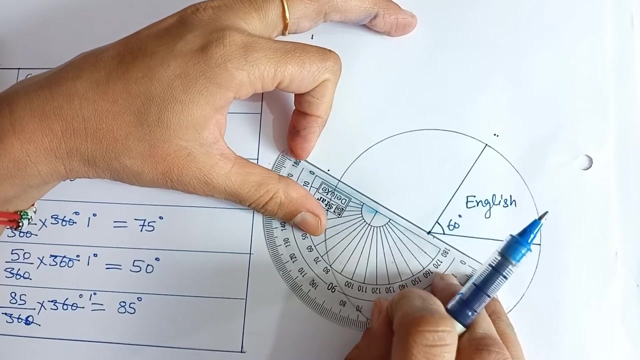 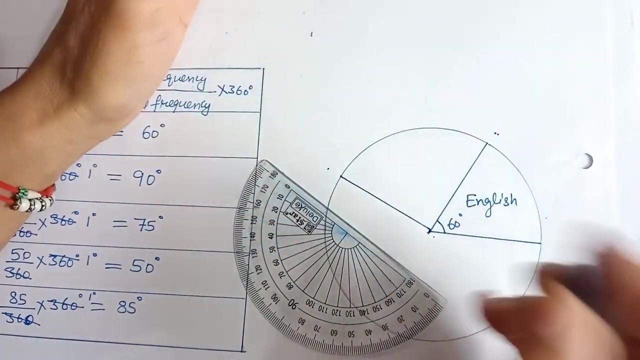 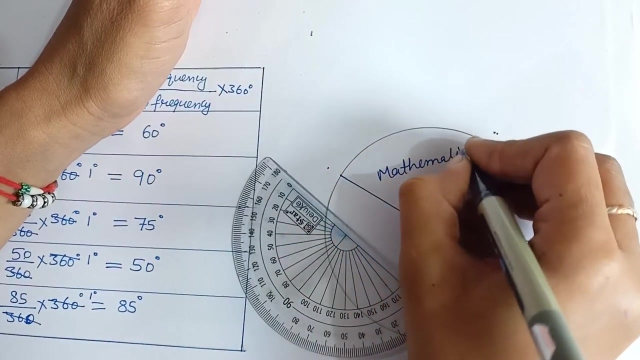 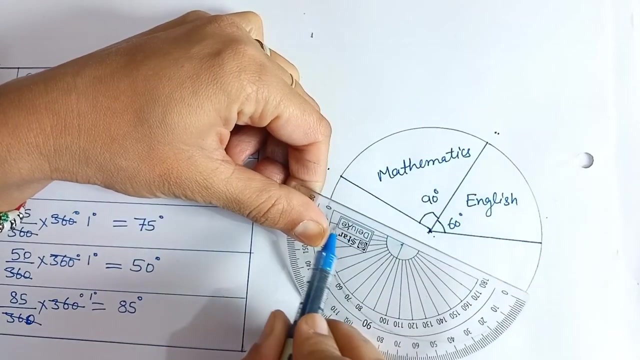 And calculate 90. Here it is 90. Then center to this point gives 90 degree. Or you can first draw the 90 degree angle and do this. This is 90 degree for mathematics. Now, next angle is 75 degree. Again, this point must coincide: center of circle and this 0 degree line over this line. 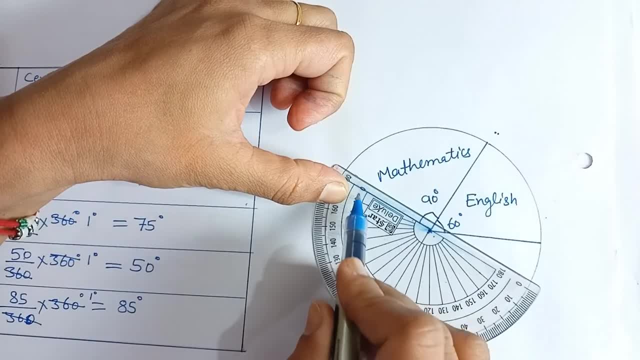 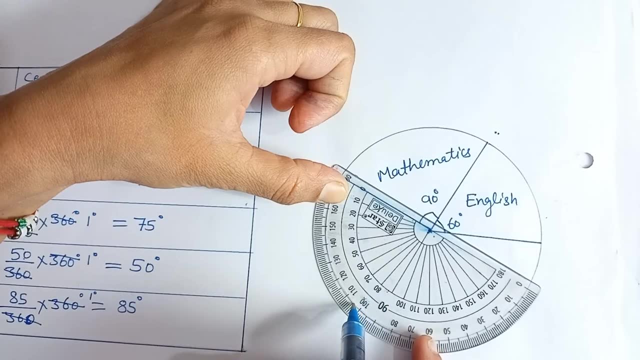 And read 75.. 0,, 10,, 20,, 30,, 40,, 50,, 60,, 70. And this is 80.. In between 70 and 80, there is a line. This is of 5..